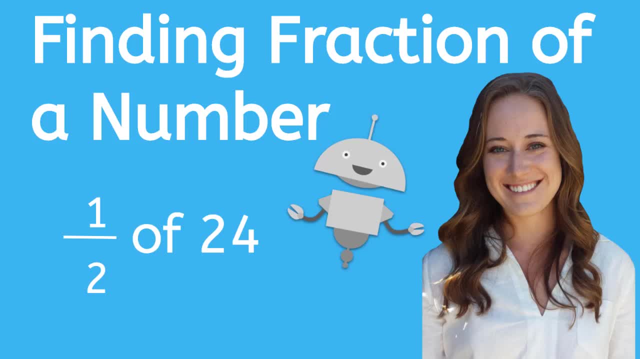 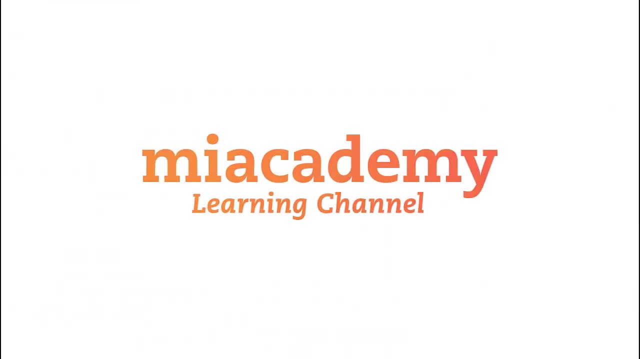 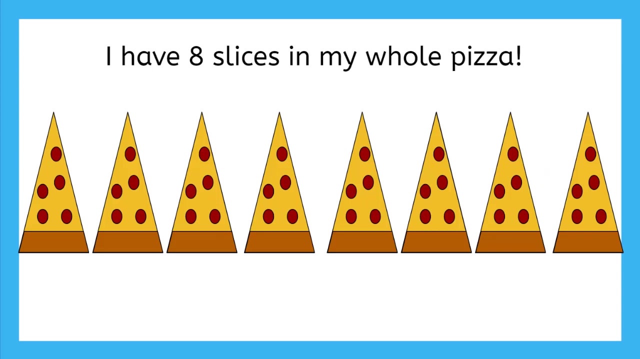 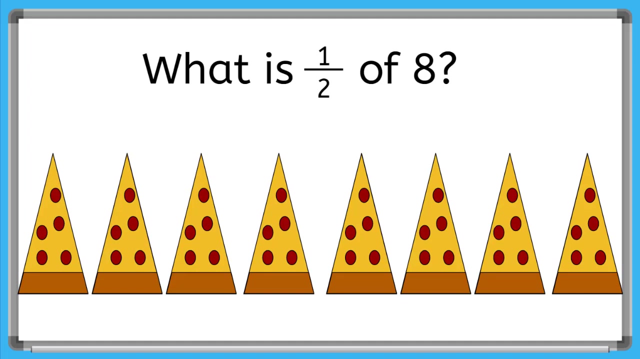 Hey, there it's Kayleigh. This lesson is on finding the fraction of a number. If I told you my pizza has eight slices and I wanted to give you half of my pizza, how many pieces would you get? So you would ask: what is half of eight? And since the fraction says one over two, 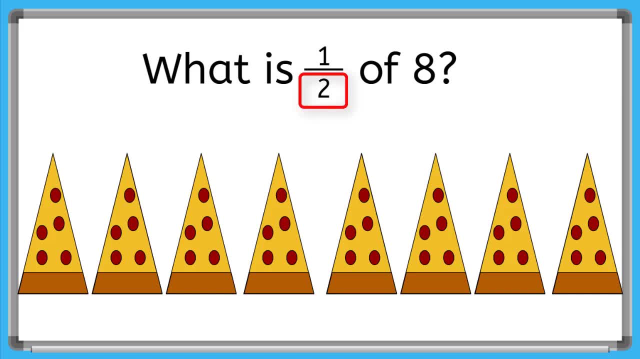 this tells me I'm dividing my pizza into two groups. Now that I've divided my pizza into two even groups, I can count how many slices are in each group. I count one, two, three, four. You would get four slices of pizza. Let's try another one. 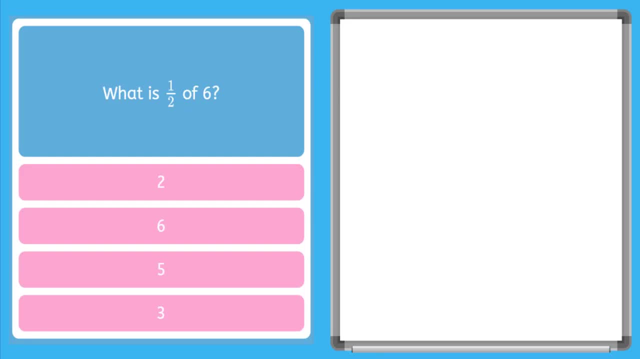 This one is asking me: what is 1 half of 6?? To help me, I am going to draw 6 candies. Now, if I look at my fraction, it says 1 over 2.. Now this says 1 over 2,. 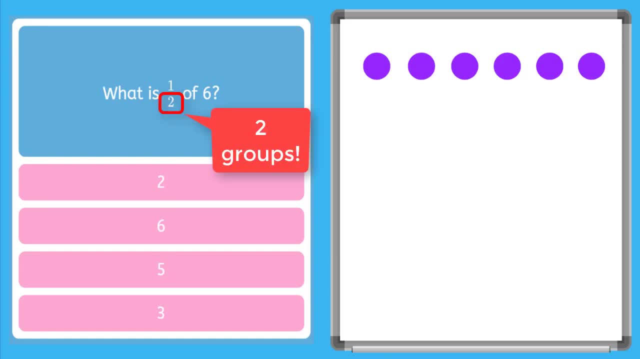 so again, this one tells me I am going to make 2 even groups with my candy. And then if I look at my fraction and I see 4 slices of pizza be throw a out, get four slicesothe pizza. This is countin this level. 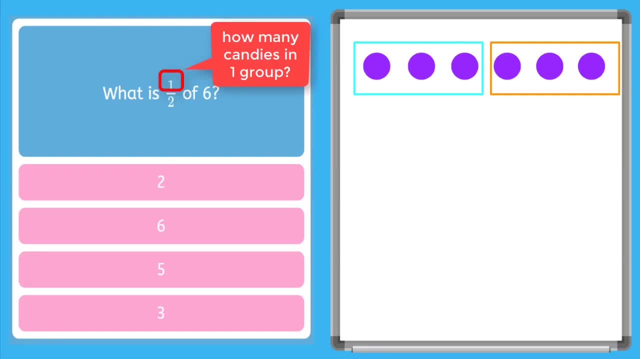 But I've got a 3, and 4 slices of pizza fraction. again, I see a one on the top. So I'm only interested in how many candies are in one group. So if I look at just one group and I count my candies, I see one, two, three. 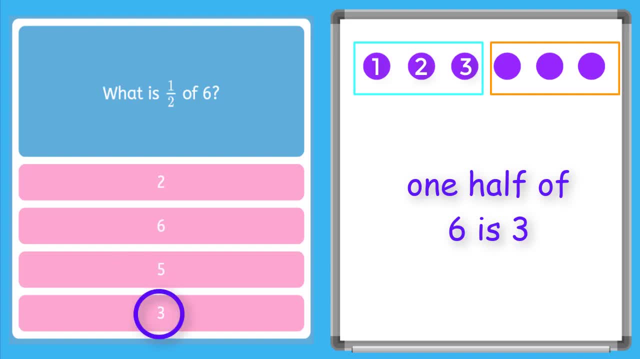 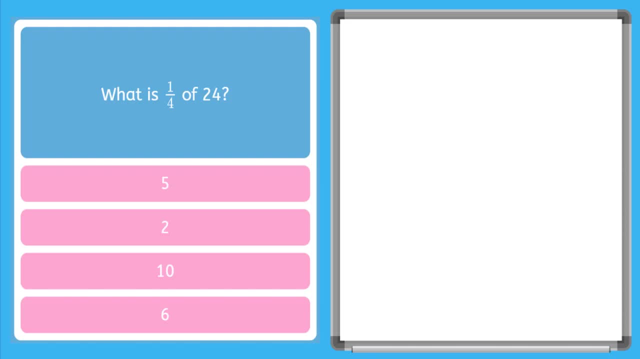 So this tells me that one half of six is three. Now let's try a harder one. This one asks: what is one fourth or a quarter of 24?? Let's draw our candies to help us think about this. Here are my 24 candies. That's a lot of candy. I can look at my fraction and it says one. 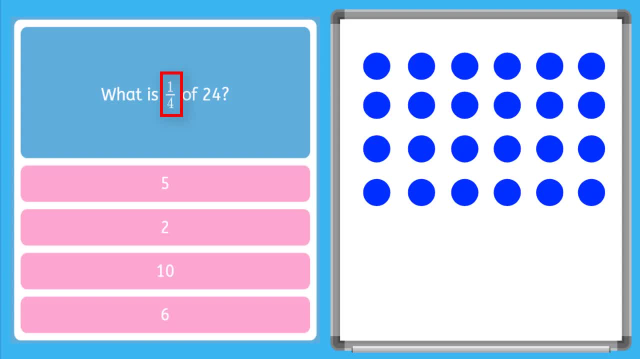 over four. So what is that asking me? Well, in real life, I could have 24 candies and four friends, And I want to give my four friends each the same number of candies. So I'm going to take my four friends and I'm going to divide them by the number of candy. So how?